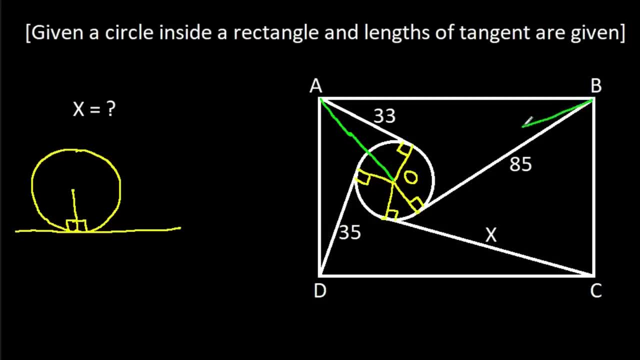 is B, So we have to find AO. this angle is O and this angle is B. So in this description BO, CO and BO. then here suppose this point is M, then interangle AOM: it is AOM, this angle is 90 degree, AM is 33 and OM it will be radius, so AOSQ. 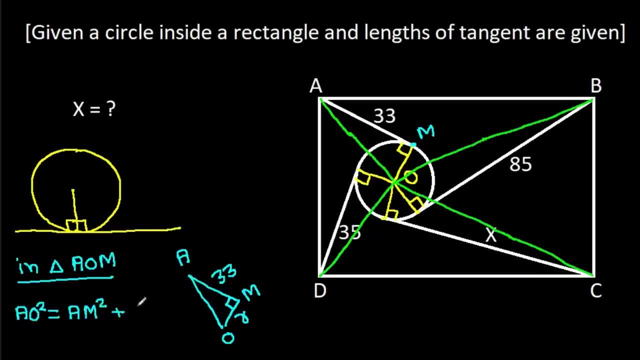 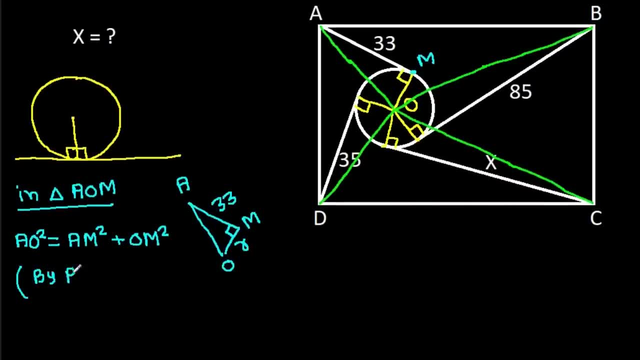 it will be AMSQ plus OMSQ By Pythagoras theorem. so we get: AOSQ is equal to AM, is 33SQ plus OM is RSQ, where R it is radius. that is, we can find AOSQ is equal to 33SQ plus OSQ, which is Om is R. 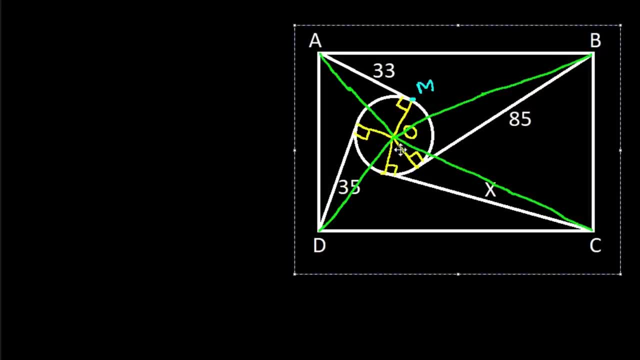 So we get: AOSQ is equal to 33SQ plus RSQ because OM is R, And in this sequence AOSQ is equal to 33SQ plus RSQ because OM is R. So we can find AOSQ is equal to 33SQ plus RSQ because OM is R. 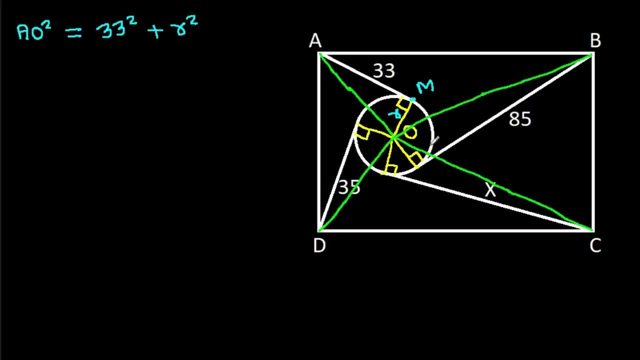 This is the starting point and in the same way, inter angle BO- and suppose this point is N- we can get BO square is equal to 85 square plus R square, because ON it will be R. and in the same way we can get CO square: it will be equal to X square plus R square and DO square it will be equal to 35 square. 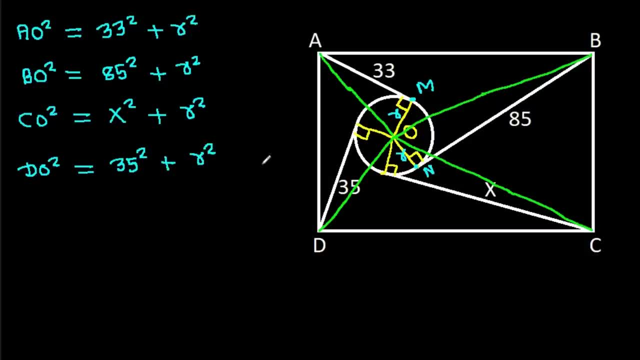 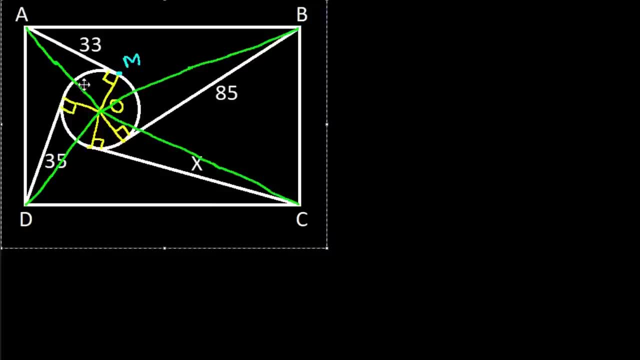 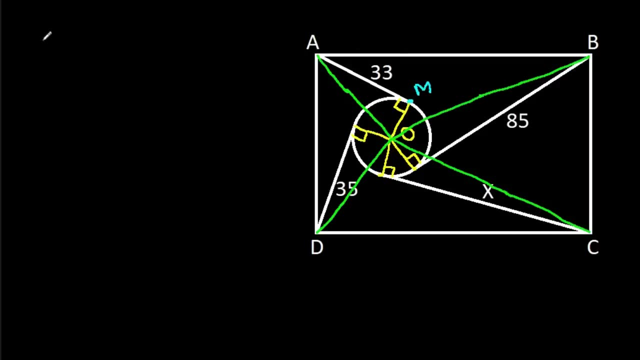 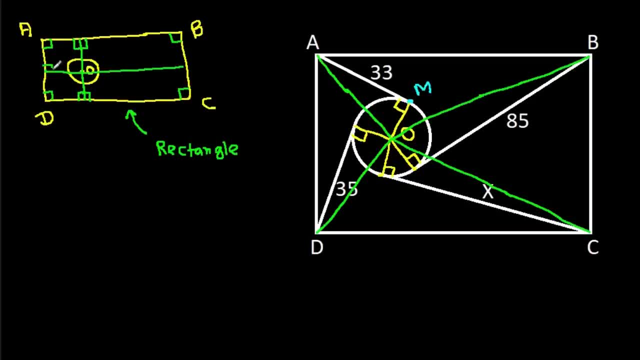 let's, let's now. And now, if AP is B1 and BP is B2, then DQ it will be also B1 and QC it will be B2.. And suppose AS is H1 and SD is H2, then PO it will be H1, OQ will be H2 and BT it will. 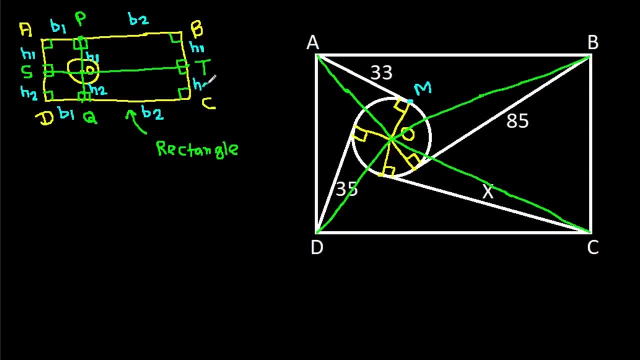 be H1 and TC it will be H2.. So if we join AO, then AOSQ will be A2.. It will be B1AQ plus H1AQ, because angle APO is 90 degree. And if we join BO, then BOAQ, it will be equal to B2AQ plus H1AQ. 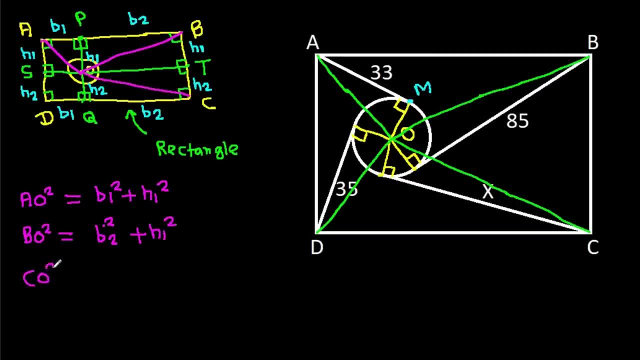 And COAQ, COAQ, IT will be B2AQ plus H2AQ And DOSQ- DOSQ, It will be equal to B1AQ plus H2AQ. So let's start. COA, COAQ- B1AQ. 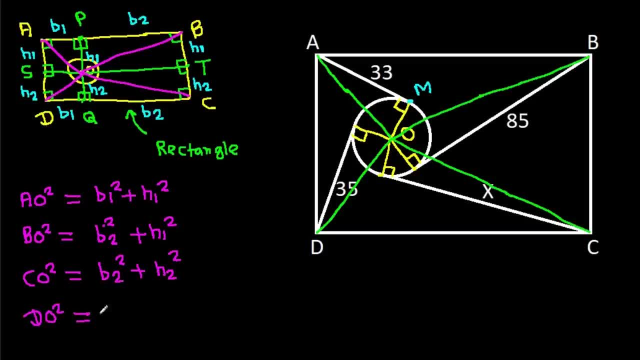 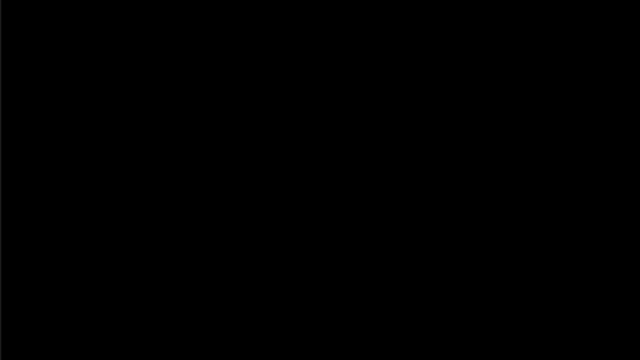 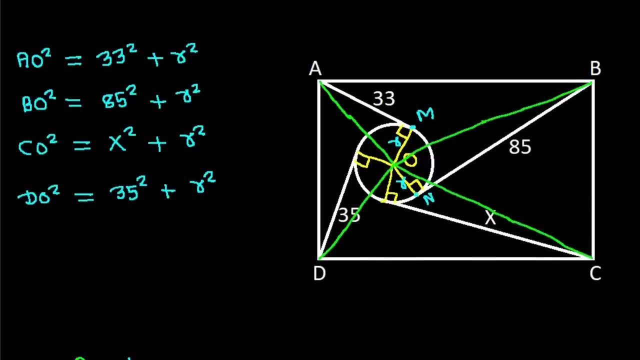 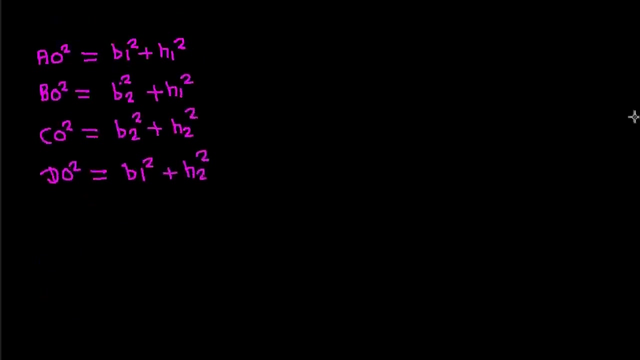 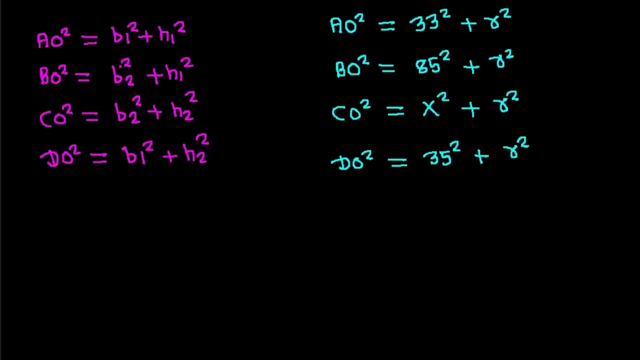 COAQ, COAQ, COAQ. We have these four equations and also, we have these four equations and now, if we compare these equations, then A O square, it is B1 square plus H1 square and A O square it. 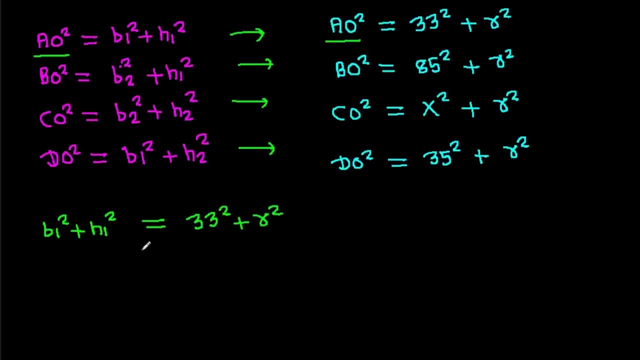 is 33 square plus R square and B O square. it is B2 square plus H1 square, and B O square is also equal to 85 square plus R square and C O square. it is B2 square plus H2 square. 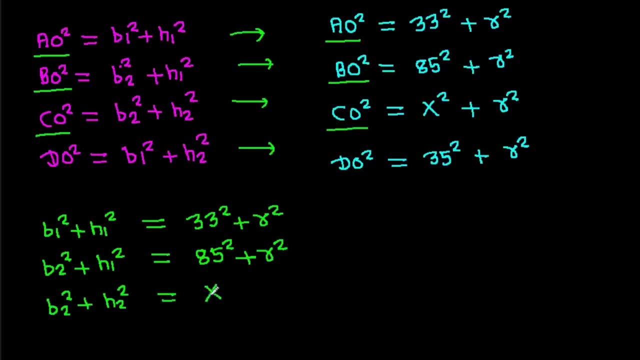 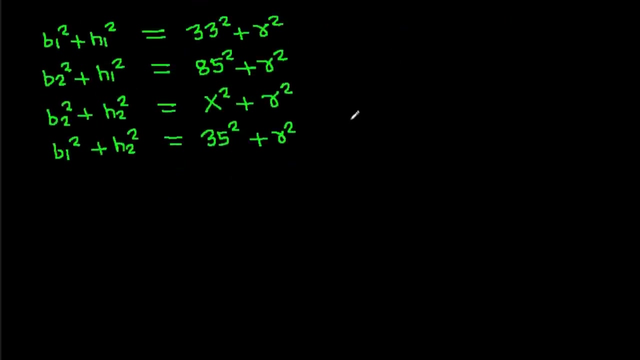 and C O square. it is also equal to X square plus R square and D O square. it is B1 square plus H2 square and D O square. it is also equal to 35 square plus R square. so now we. 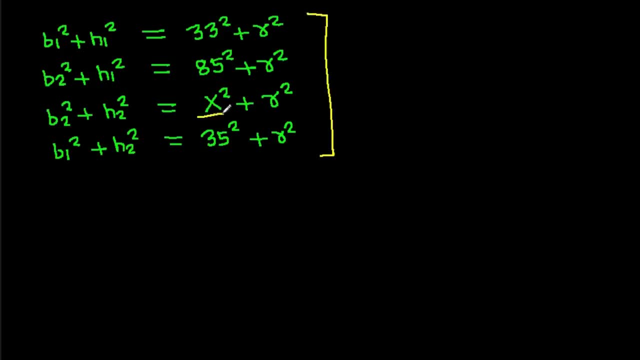 have four equations and we have to find X. So suppose this is equation 1.. this is equation 2, this is equation 3 and this is equation 4. and now if we subtract equation 1 from equation 2, equation 2 minus equation 1, then it will. 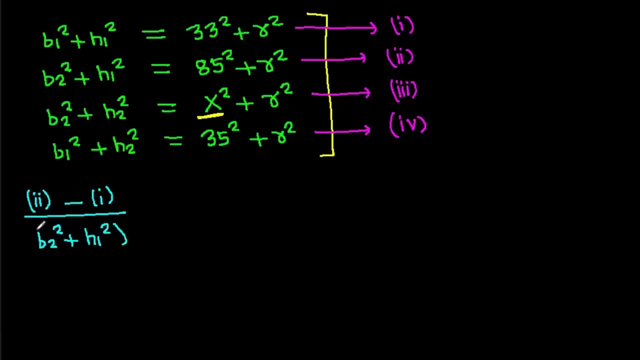 be b2 squared plus h1 squared minus b1 squared plus h1 squared is equal to 85 squared minus r squared minus 33 squared minus r squared and h1 squared will get cancelled, and here r squared will get cancelled, so we get b2 squared minus b1 squared is equal to 85 squared. 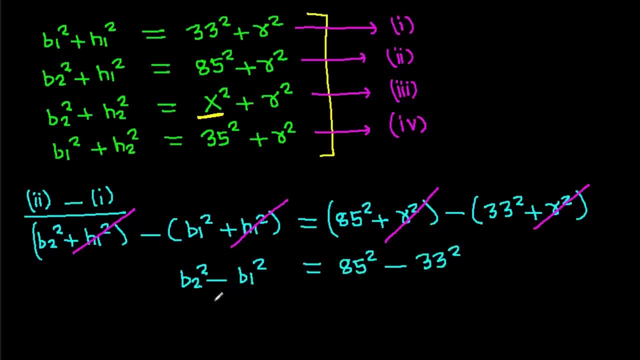 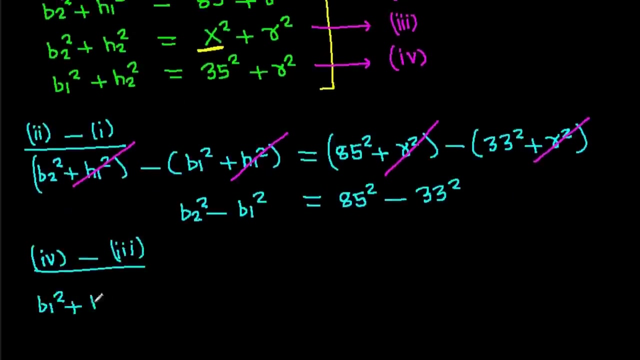 minus 33 squared. and now, if we subtract equation 3 from equation 4, equation 4 minus equation 3, then it will be b1 squared plus h2 squared minus b2 squared plus h2 squared is equal to 35 squared plus r squared minus x squared plus r squared and h2. 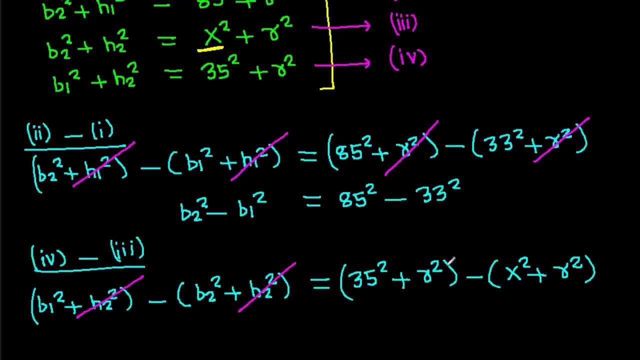 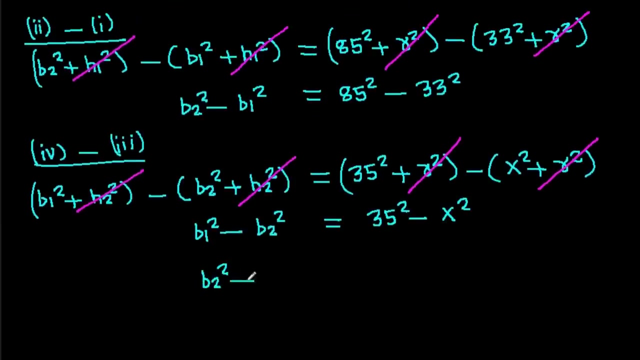 squared will get cancelled, and here r squared will get cancelled, so we get b1 squared minus b2 squared is equal to 35 squared minus x squared. so b2 squared minus b1 squared it will be x squared minus 35 squared, and suppose this is equation 5. 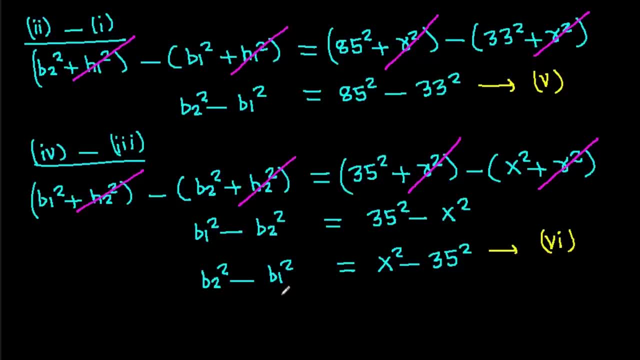 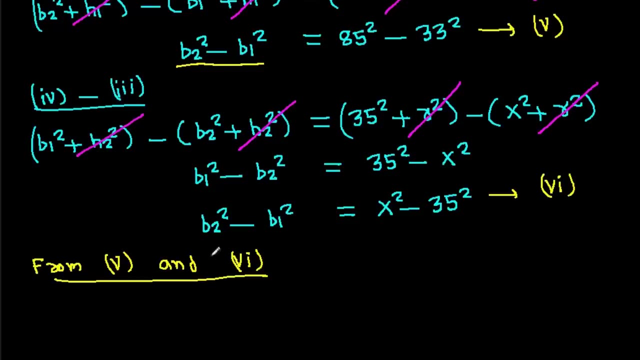 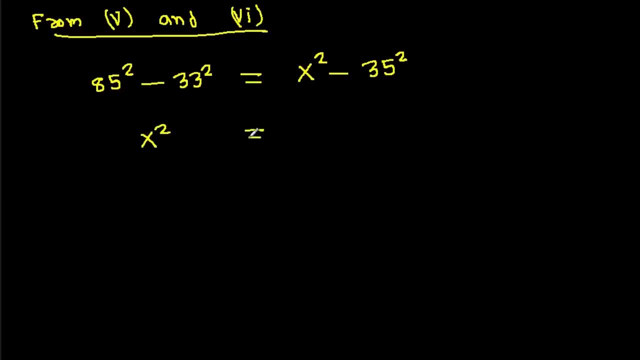 And x square, it will be equal to 85 square minus 33 square, minus 35 square, Okay. And x square, it is 85 square minus 35 square, minus 33 square. And x square, it is equal to and a square of any number. suppose x ending with 5, it. 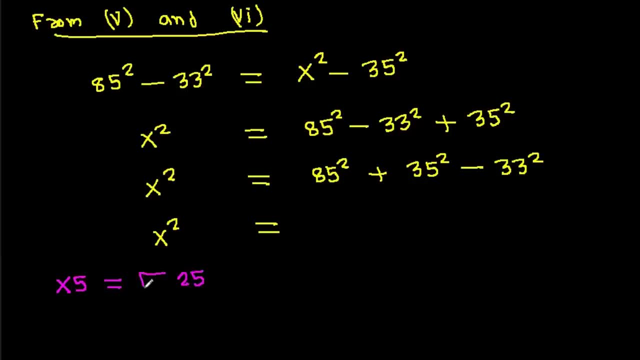 will be 2, 5 at the end. And here, For example, it will be x times x plus 1.. For example, 45 square, it will be 2, 5 at the end. And 4 times 4 plus 1 is 20, 65 square, it will be 25 at the end. 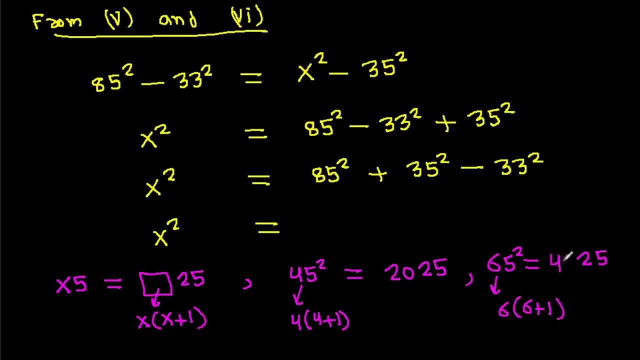 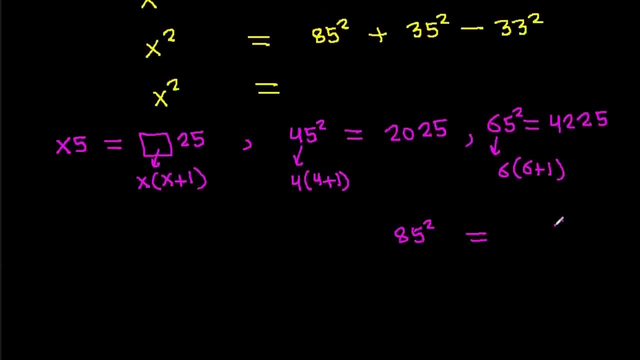 And 6 times 6 plus 1, it is 42. So Okay, So 85 square, it will be 2, 5 at the end, And 8 times 8 plus 1, it is 8 times 9, that is 72.. 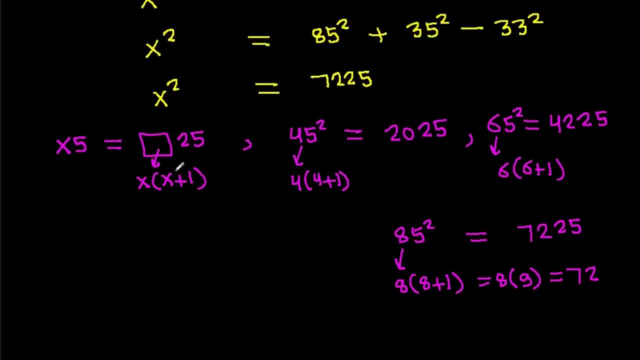 So it will be 7, 2, 2, 5.. And we know that a square minus b square minus 3 square minus 3 square, it will be 7, 2, 2, 5.. And 8 times 8 plus 1, it is 8 times 9,, that is 72.. 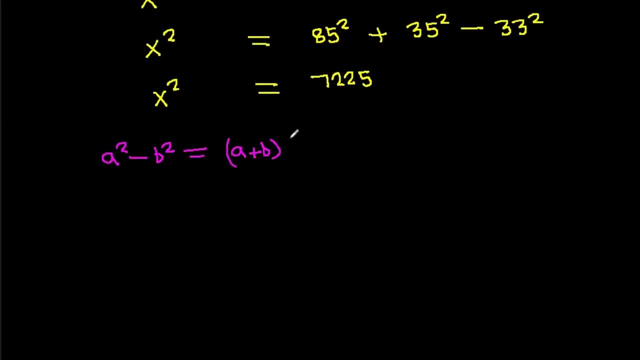 So it will be 7, 2,, 2, 5.. And we know that a square minus b square is a times b times a minus b. So 35 square minus 33 square, it will be 35 plus 32 times 3, 5 minus 33.. 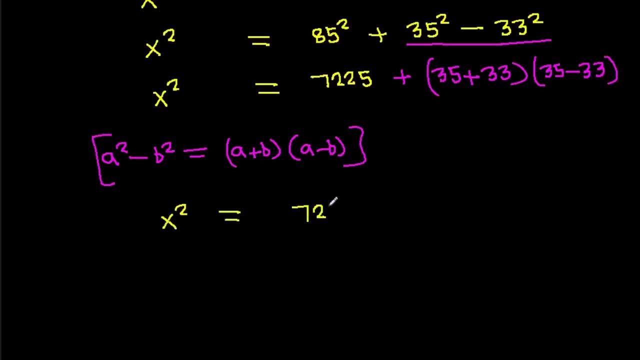 So x square, it is 7225 plus This will be 68.. Okay, times 2 and x square, it is 7225 plus 68. times 2, it will be 136.. So we get: x square is equal to 5 plus 6 is 11 and 2 plus 3 is 5 plus 1 is 6 and 2 plus. 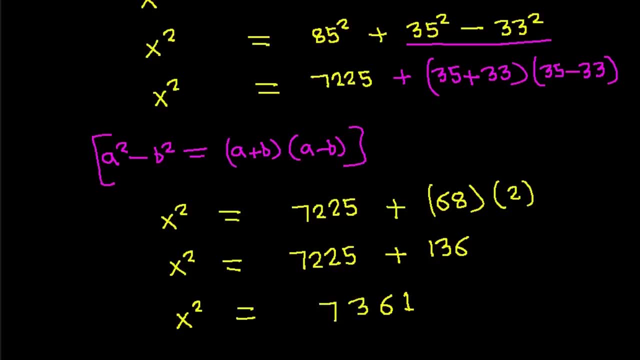 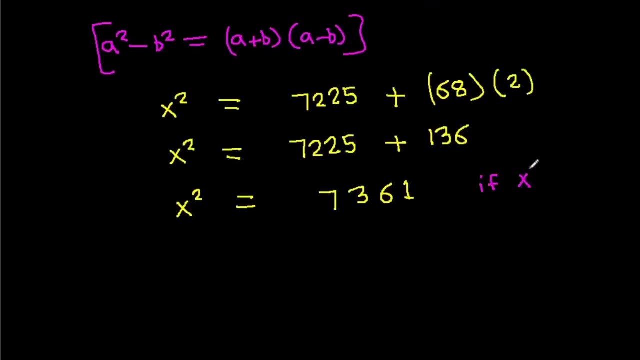 1 is 3 and 7. And if we have x square is a, Then x square is a, Then x will be equal to minus minus a square root of a. So x will be equal to minus minus a square root of 7361.. 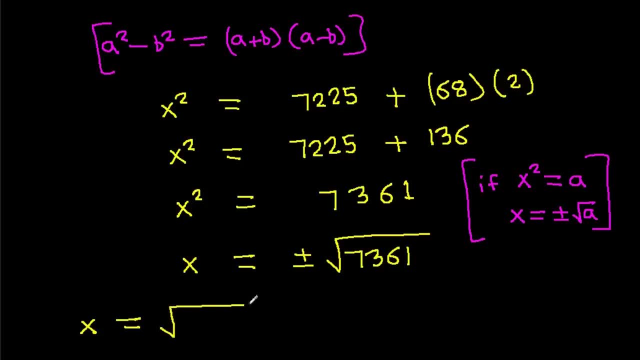 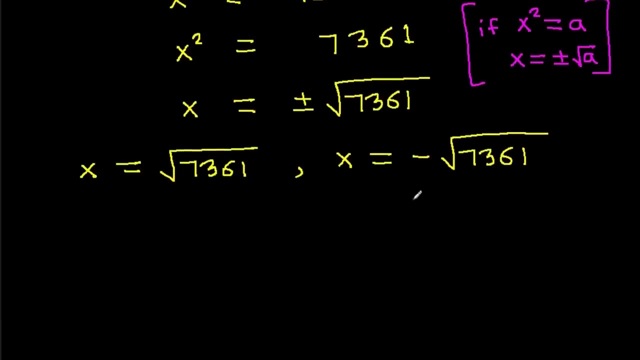 So we get: x is a square root of 7361 and x is equal to minus a square root of 7361.. But x is length. that should be positive. So x cannot be negative. So x will be equal to a square root of 7361.. 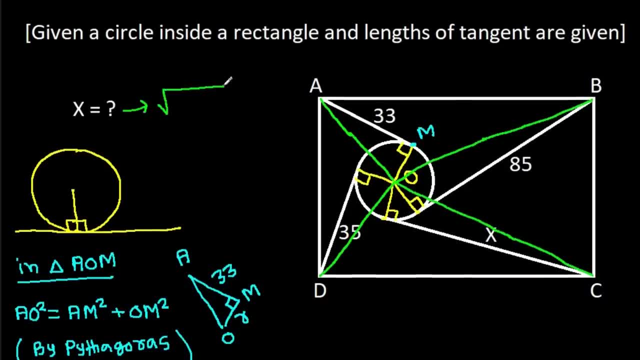 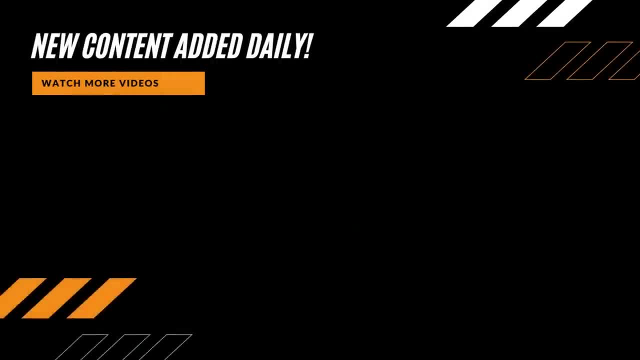 x is a square root of 7361.. 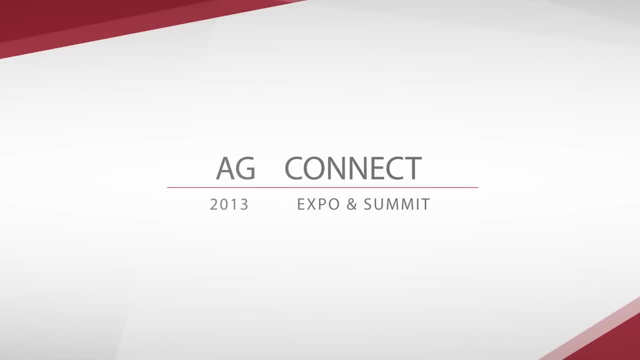 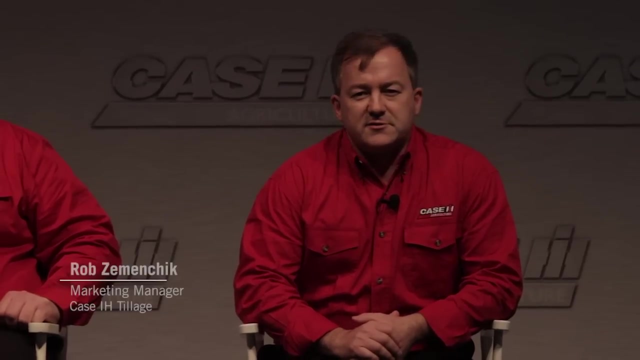 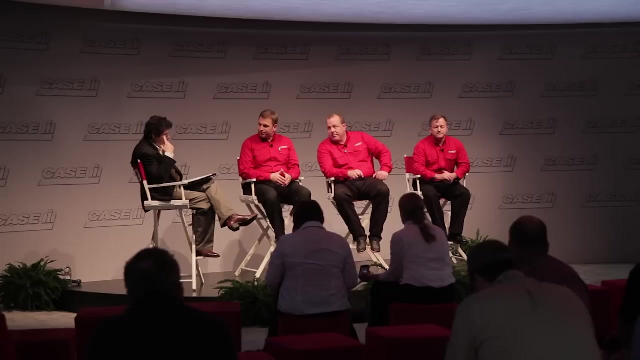 Soil compaction is really the absence of pore space and the eradication of soil structure. It has a great effect on soil-plant-water relationships and can affect yield potential in any field. Well, when I think of soil compaction, Rob, one of the first things that come to.